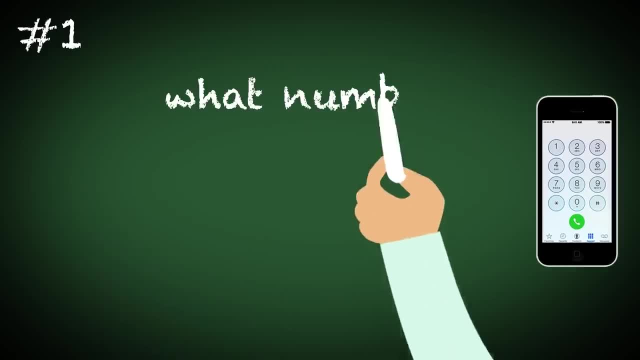 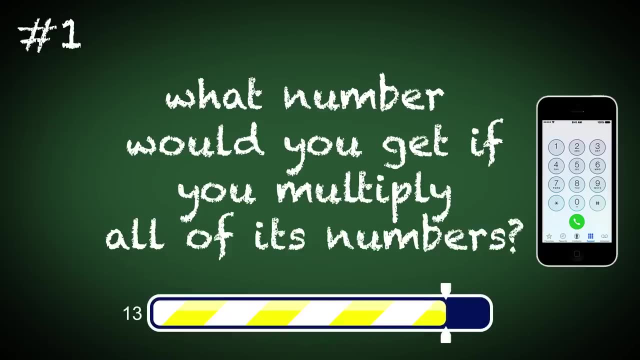 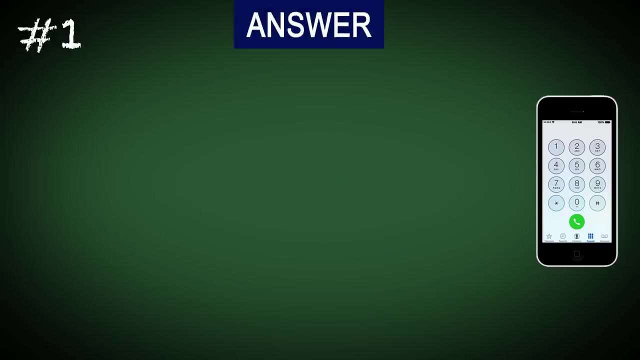 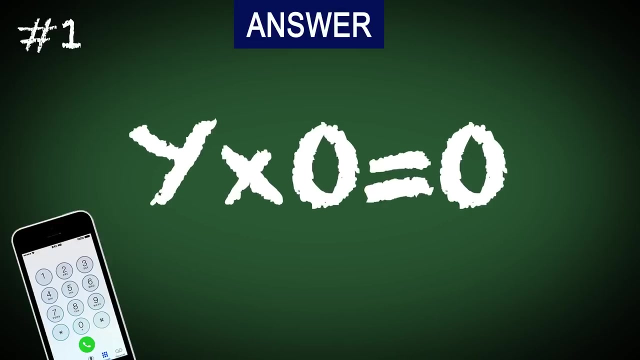 a look at your telephone's number pad and answer this: What number would you get if you multiply all of its numbers? You have some time to count. Here's the answer. You didn't forget about zero, right? Whatever is multiplied by zero will give you zero. This golden rule of math always works. 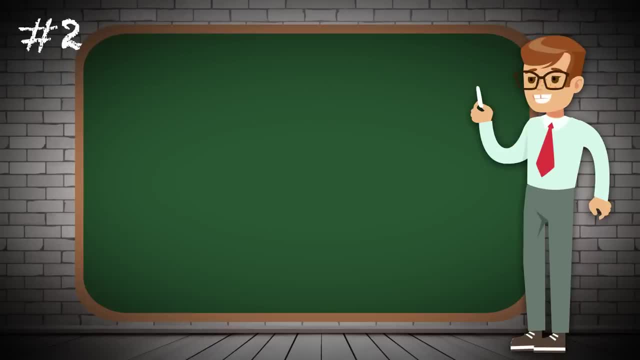 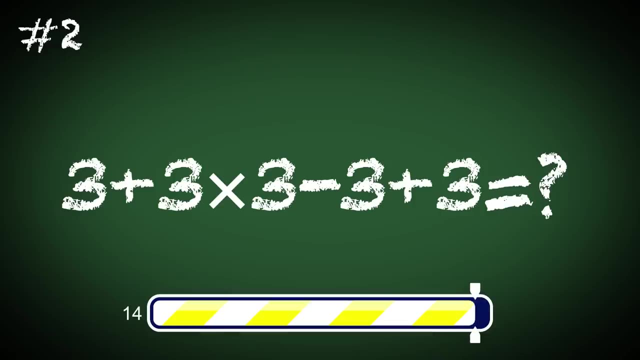 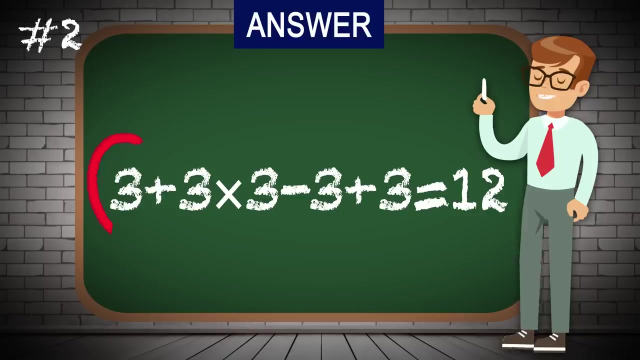 Number two: Find a correct answer to this math equation: Three plus three times three minus three plus three, And time is over. If your answer is 12, you're out Absolutely right. Three plus nine is 12.. 12 minus three plus three is still 12.. Let's see how you. 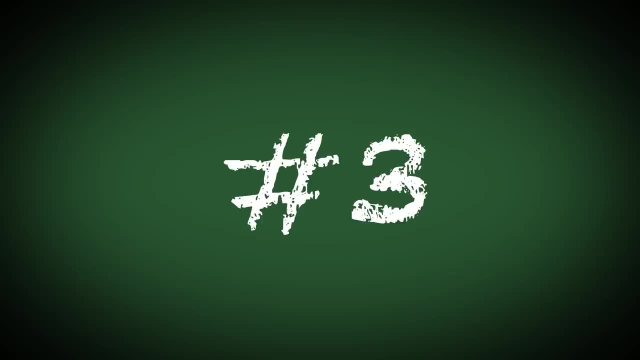 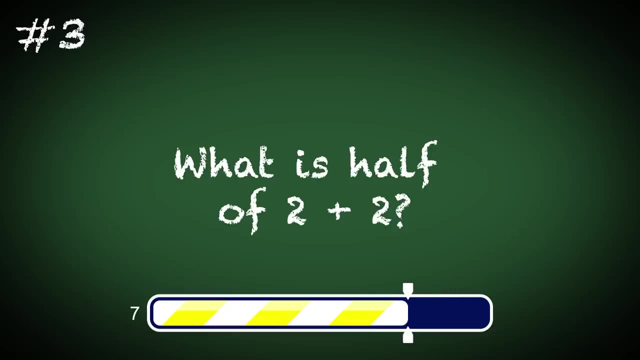 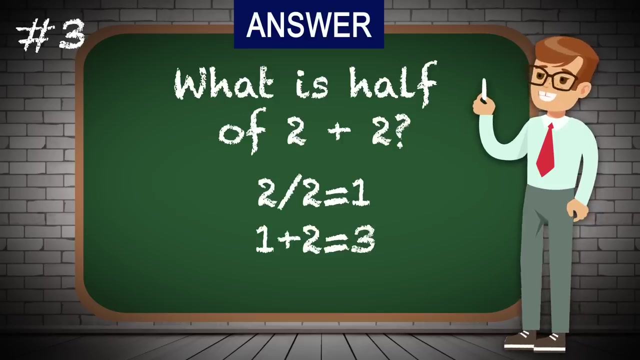 pass our next question, Number three: What is half of two plus two? Time is ticking. It's not two, but three. Half of two is one, and half of two is two, And one plus two is three. Nice and easy, Yeah. 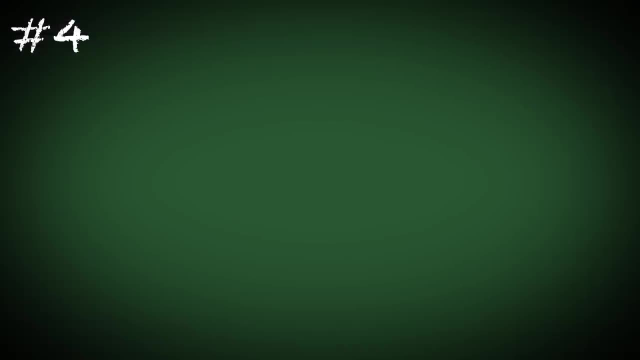 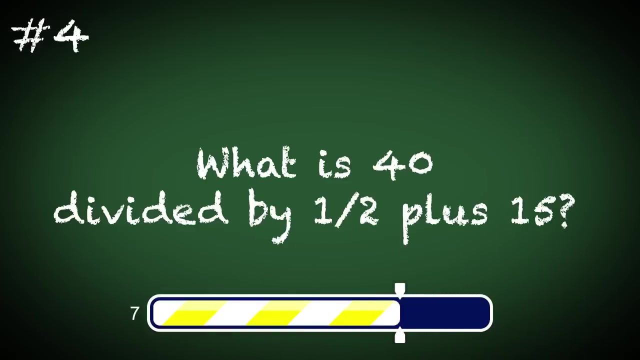 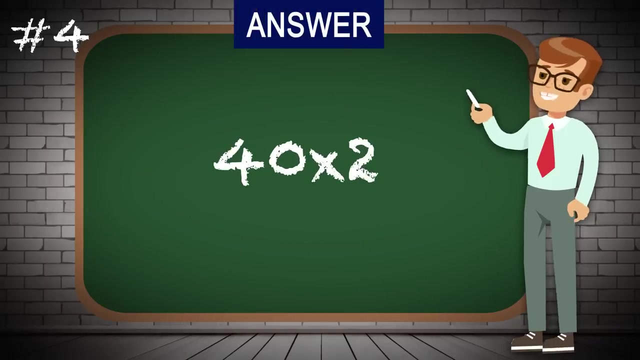 Number four: Just a simple math question for you. What is 40 divided by one-half plus 15?? Dividing by one-half is basically multiplying by two, remember? No, I really don't, Anyway. so 40 times two equals 80.. 80 plus 15 is 95.. Props to you if you didn't get. 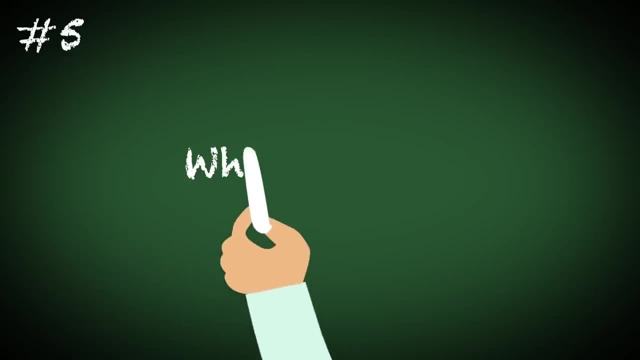 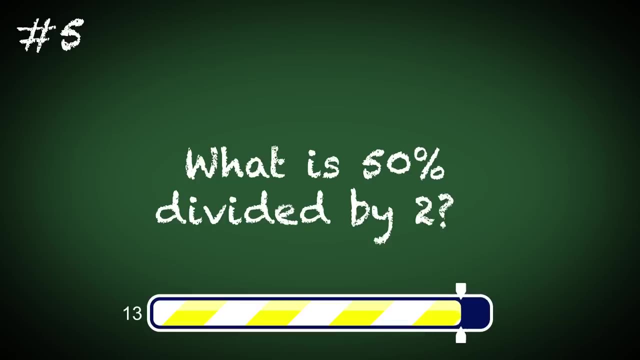 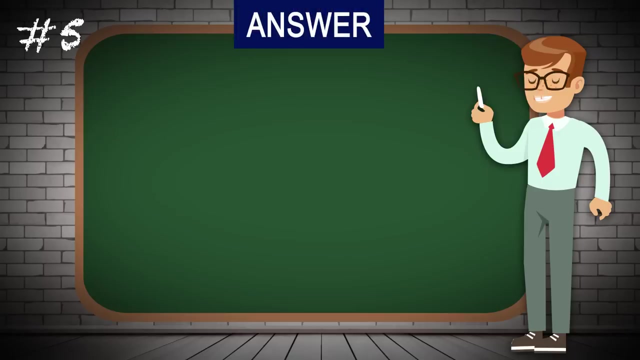 distracted Number five: What is 50 percent divided by two? You have 15 seconds to prepare your answer. It's actually just 1.. You have to think outside of the box for this one. 50% is one half right. 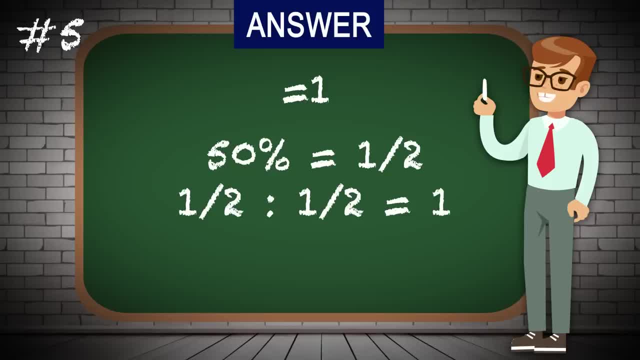 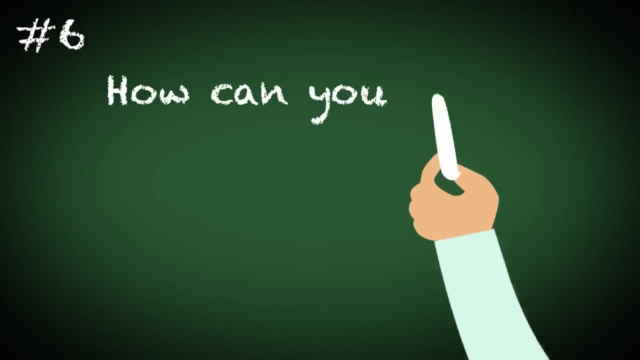 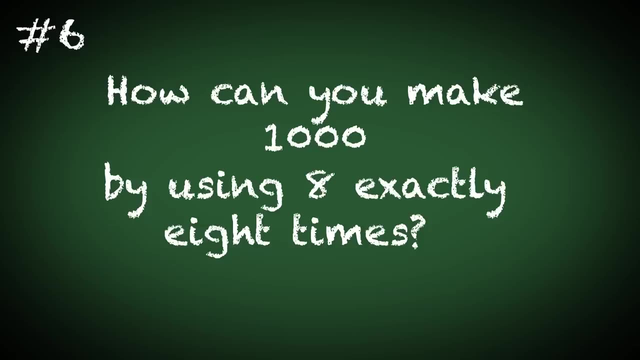 One half divided by one half will give you 1.. Did you get it? Well, pull yourself together. the next question is coming, Number 6.. How can you make 1,000? by using 8, exactly 8 times. Keep in mind that you can only use addition in your equation. 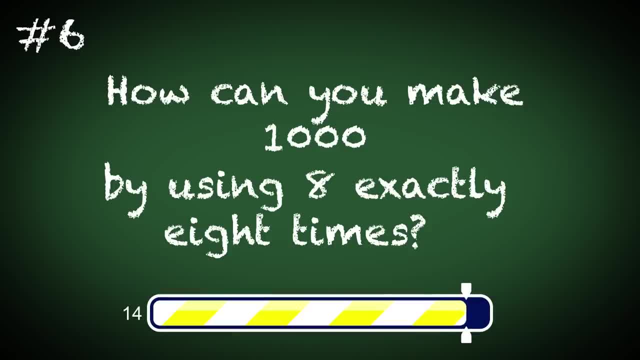 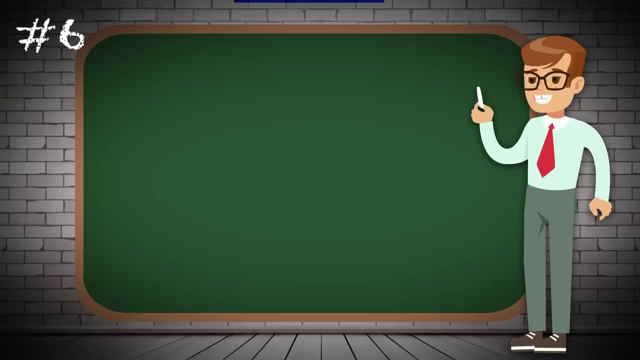 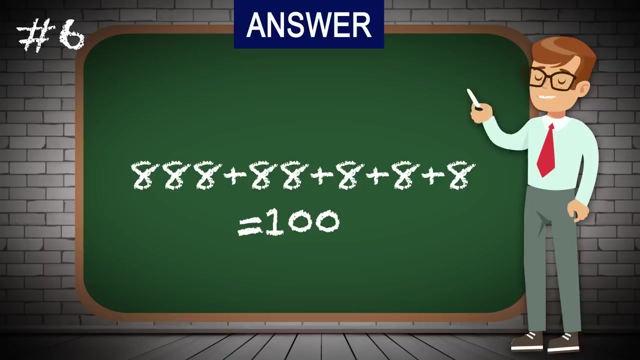 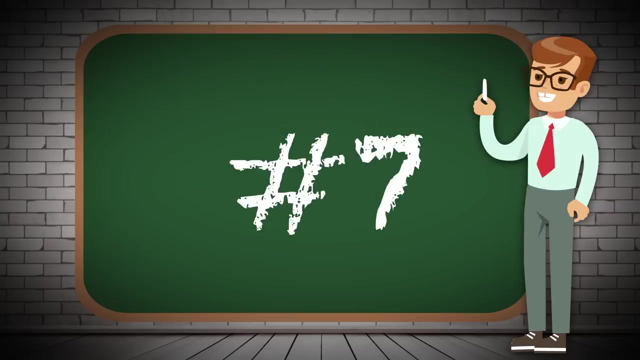 Try to come up with the answer in 15 seconds. The right equation is 888 plus 88 plus 8 plus 8 plus 8 equals 1,000.. Do you have a different but still correct answer? Share it in the comments below. 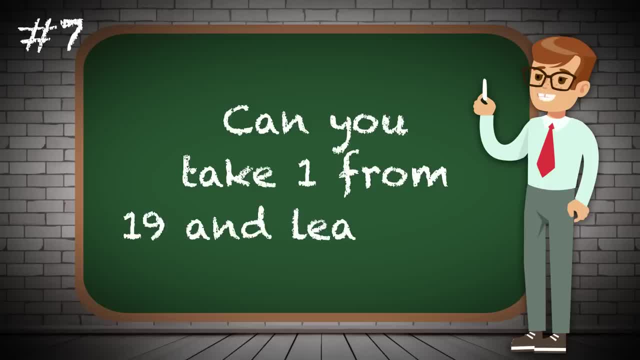 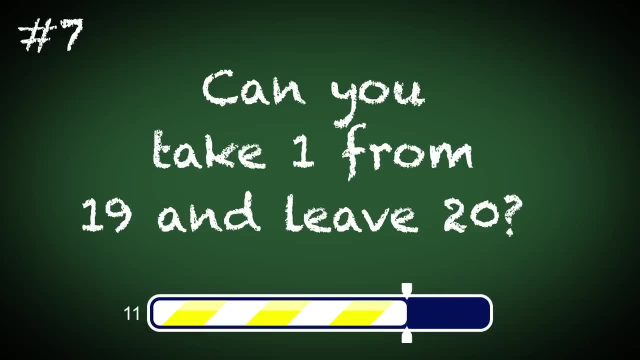 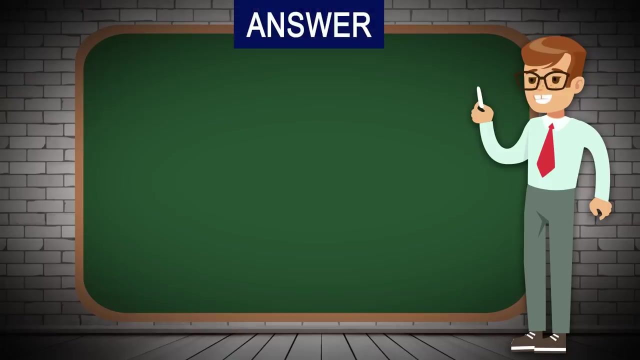 Number 7.. Can you take 1 from 19 and leave 20? You have 15 seconds to figure out a way. You can easily do it with 4.. 5. You can easily do it with roman numerals: 20 is xx, while 19 is xix. 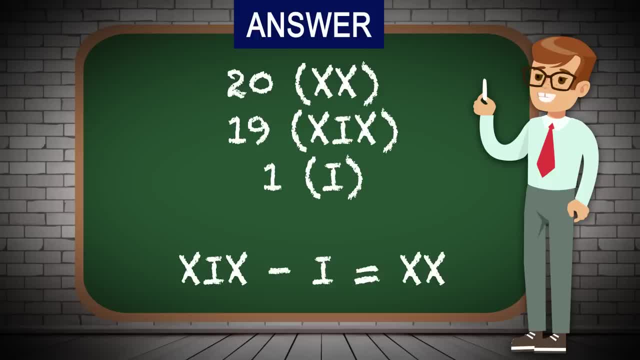 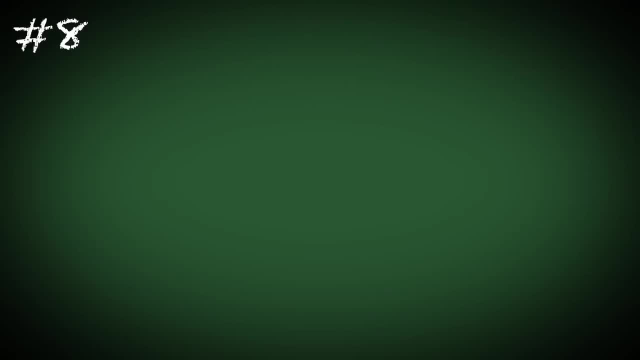 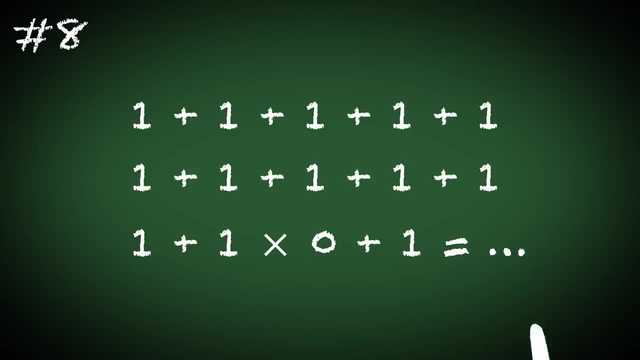 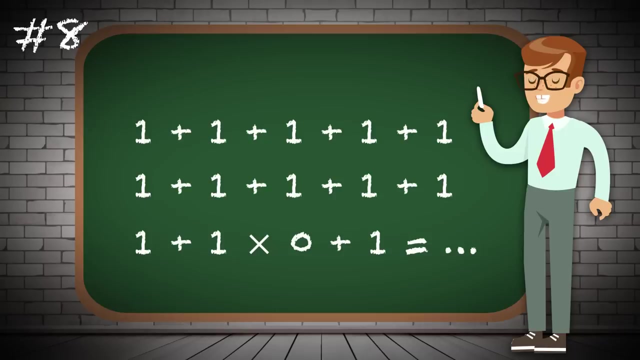 1 plus 1 multiplied by 0 plus 1 equals 1.. Are you ready? Equals… Can you solve this? You have 15 seconds. No, the right answer is not 1, and it's not 12 either. It's actually 2.. 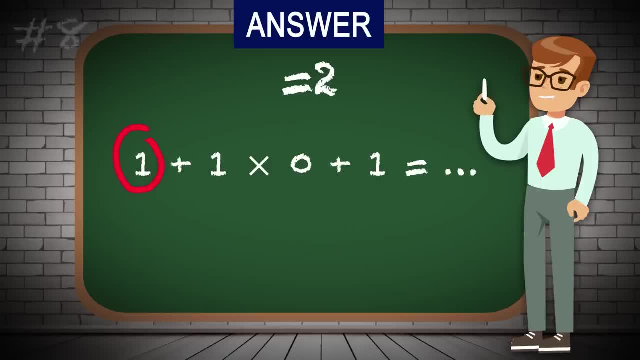 The first two lines aren't part of the equation. So 1 plus 0 plus 1 gives us 2. as a result, You know, I had a math teacher like this, Vicious woman. vicious woman, Number 9.. So pay attention. 1, 1, 1, 2, 1, 1, 2, 1, 1, 1, 1, 2, 2, 1, 3, 1, 2, 2, 1, 1..